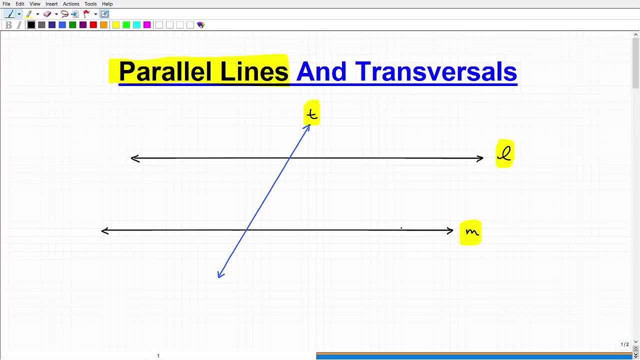 based upon the way a figure looks, that two lines are parallel. you have to actually very specifically state that. so the ways we can do that is we could say L is parallel to M, line L is parallel to M. that's one way of doing it. another way you can do it is: you can see a another arrow here on the line and you 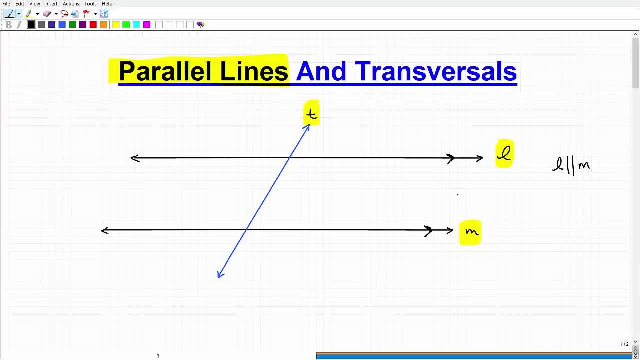 put another one down here. okay, so this indicates that these two lines are parallel. without these, this notation or this notation, we cannot you assume that these two lines would be parallel. now, everything I'm going to talk to you about here- and I'm getting to transversals in a second- depends upon: 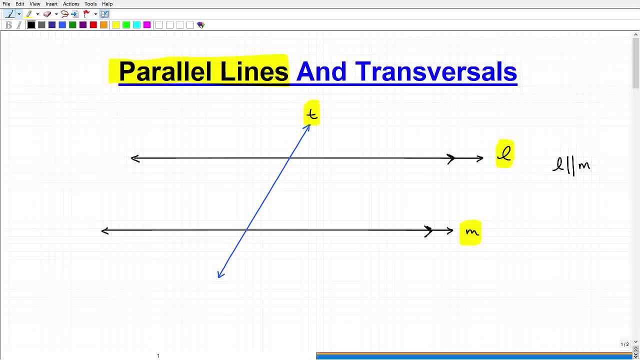 these two lines in fact being parallel, then there's a whole range of properties that that follow from that. but tests like the SAT and SAT ACT, they like to kind of quiz students. sometimes they'll draw a figure that the lines look parallel, but in fact they didn't state that. then students kind of assume well, 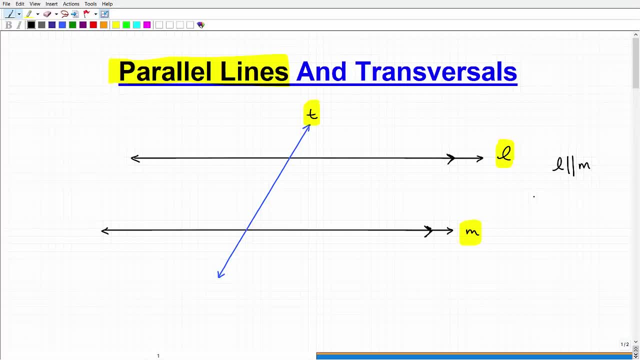 those are parallel lines. they'll work it out and they'll get the problem wrong, and they're kind of set up that way. so just be careful, right? so, um, you kind of in fact look to see that the lines are in fact stated parallel. now let's get. 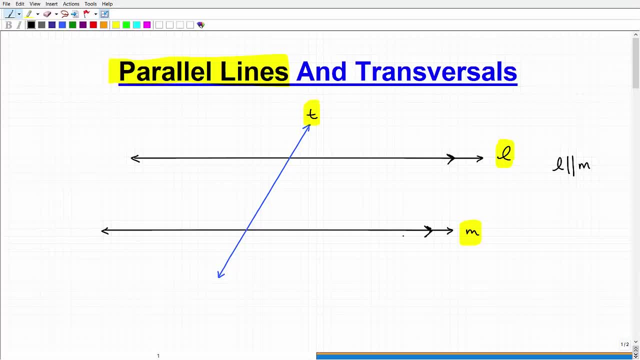 let's get into this little bit further. so if you have two parallel lines- two or more in fact, but we're just gonna stick with two- and you have another line that kind of crosses through it, like our line t here, this line T would be referred to. 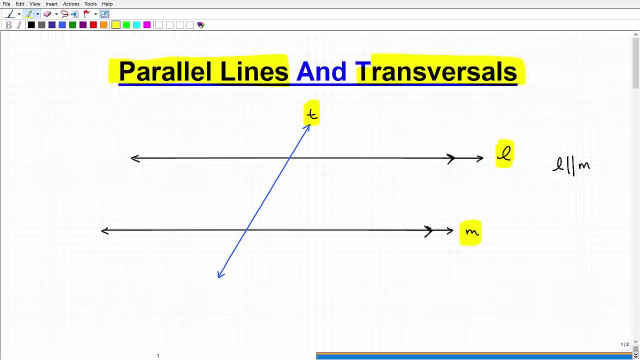 as invulnerable coating transverse pressure. so parallel line A and parallel line B are non-transverse Х and at delta P, ganska caused as a transver s Basic Special Assessment, Instagram Line T. here this line T would be referred to as a transversal. okay, so parallel line A. 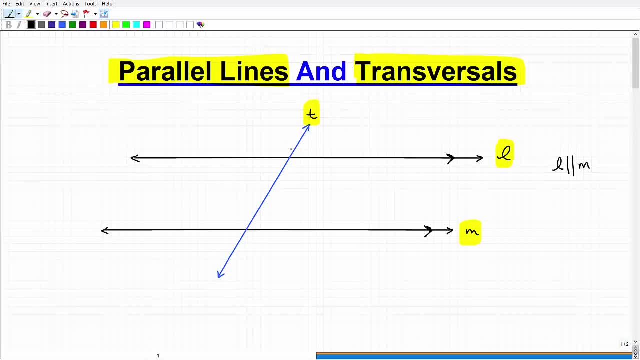 and transversal, and you can have one or more transversals. we're just gonna stick with one here now. in this case, if you have parallel lines and a transversal- and this is the most basic setup here a lot of neat properties take care of- or 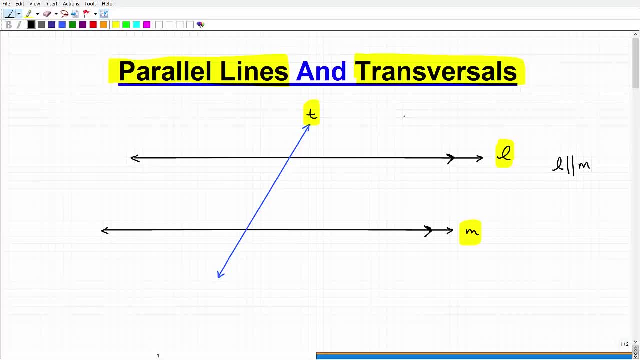 kind of come into play, and these are actual angle relationships. so let's go and just talk about a whole bunch here. it's something that you absolutely need to know and there's a lot of problems, in other words, like on your final exam, your chapter test or SAT, ACT, GED, whatever the case is that are that I'm 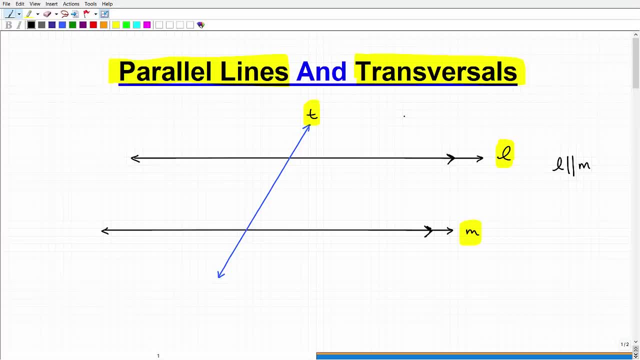 sure, going to in fact test you on your knowledge of these angle relationships. they're not hard, but there are many, okay. so I'm gonna kind of go through these and I'll race and we'll just, you know, kind of go through them one by one. so 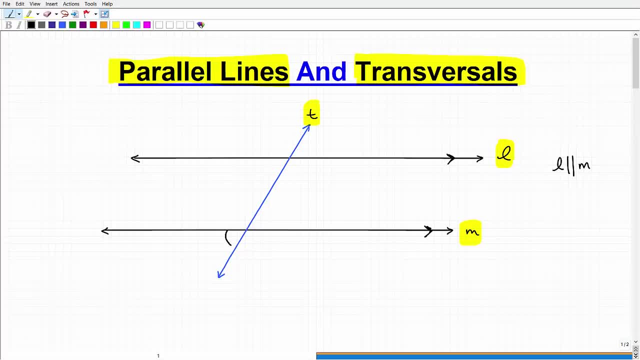 the first are vertical angles. so this angle and this angle here- okay, if you kind of look to kind of look the same, well they are, they're called vertical angles. okay, now, there are many pairs of vertical angles here. right, this here and this here there's another pair of vertical angles, vertical. 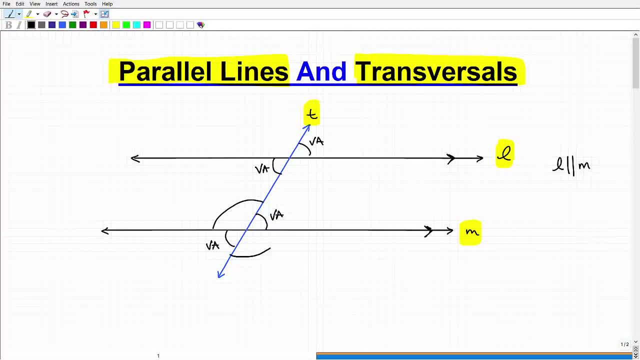 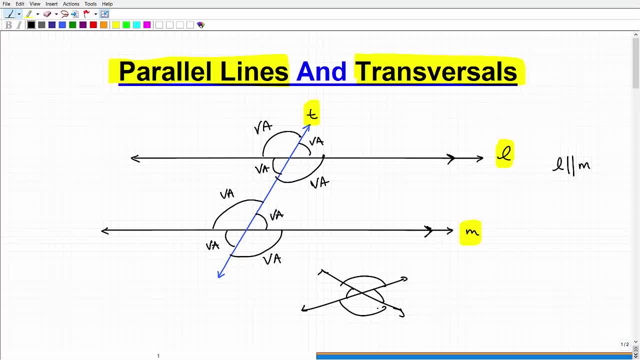 these are, vertical angles are formed okay, and vertical angles are congruent. now, the word congruent just means that they're equal, so all these angles here would be equal to one another. so we can kind of specify that and actually what i'm going to do. you're going to do it this way. 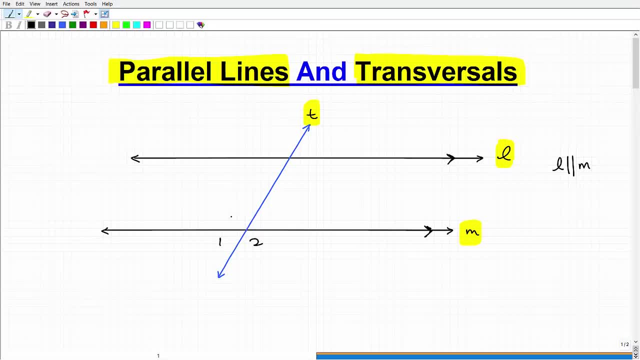 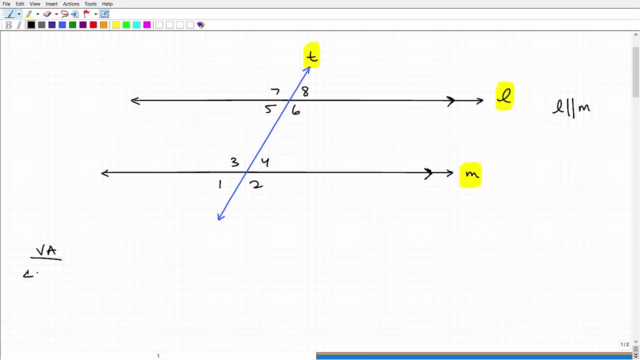 we'll give these angles some names: one, two, three, four, five, six, seven, eight. okay, so let's kind of just kind of go down here. we'll say vertical angles. where are vertical angles? angle one and four right. so angle one is congruent to angle four. why are these two angles equal to one another? 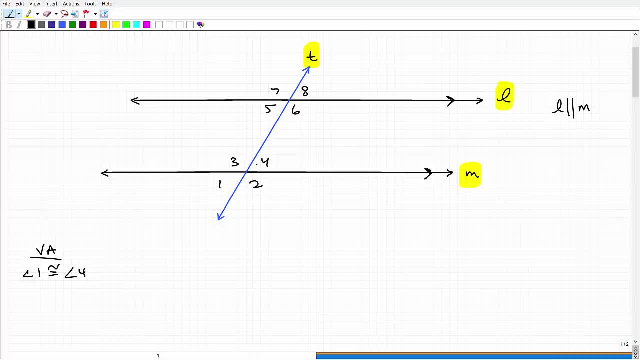 because they're vertical angles. so in geometry, mathematics, you have to have a justification. you just can't be like: well, they kind of looked like they're equal. no, well, in fact they're vertical angles. that's why they're equal, and so we can list the rest of them real quick. angle. 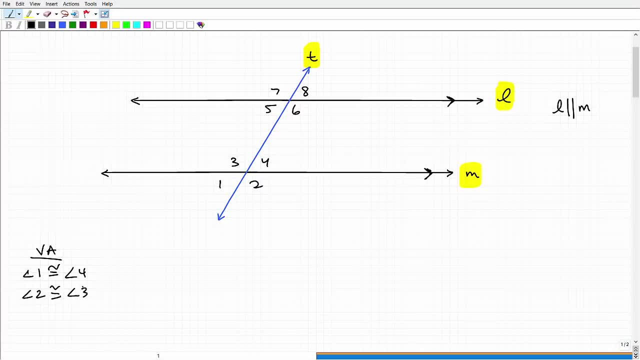 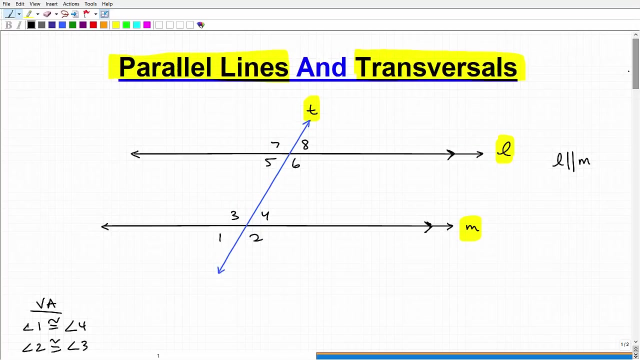 2 is congruent to angle 3, and we'll just do the rest here real quick. 5 and 8: angle 5 is congruent to angle 8 and angle 7 is congruent to angle 6. okay, so those are all vertical angles. now let's move on to some other I'm gonna get into. 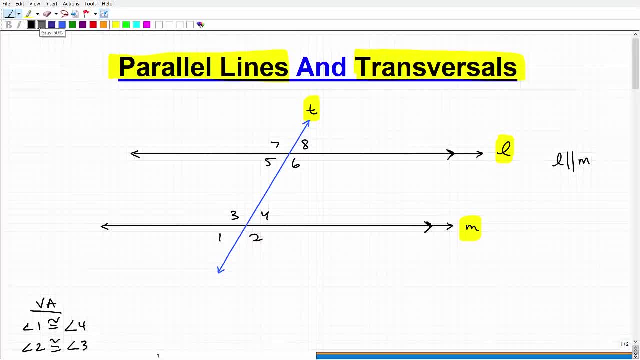 some things like alternative angles, all that stuff. maybe if you're watching this video, you probably already know a little bit about that. what kind of hold on? let's kind of take care of some of the more fundamentals. so the vertical angles are fundamentals. now straight lines are also considered angles, so like angle 3. 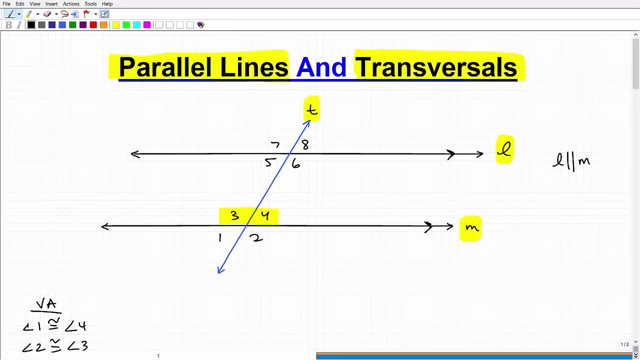 and 4, so what we call a straight line. okay, they're also supplementary, which means they add up to 180. okay, they're also supplementary, which means they add up to 180. so from here you might say: well, this is an angle, because there's like a bend in. 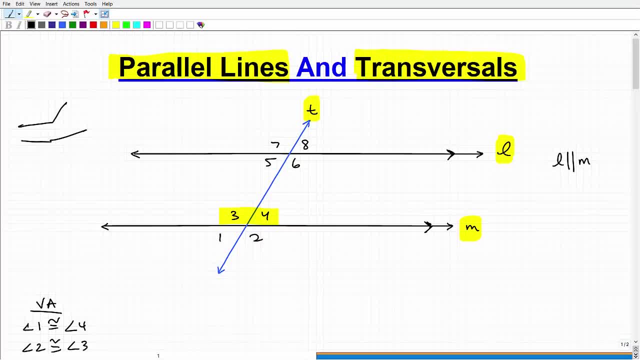 it right. well, what if I happens, if I just can't keep opening that bend up more and more and finally I open it up all the way? there's a straight line. you might be saying yourself: well, the angle disappeared. well, no, the angle didn't disappear. there's still an actual angle here. right, the angle of a straight line. 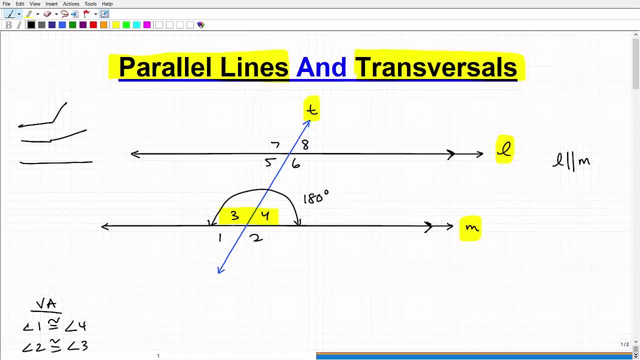 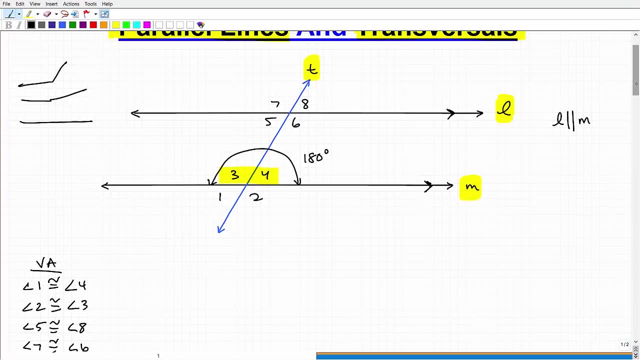 is 180 degrees. okay. so any two angles that make up if you add them, or basically are adjacent, that add up to 180 degrees, now they form a straight line angle. okay, they're also supplementary, so we can kind of build out some additional angle relationships here. so let's kind of do this here. so let's say straight line for. 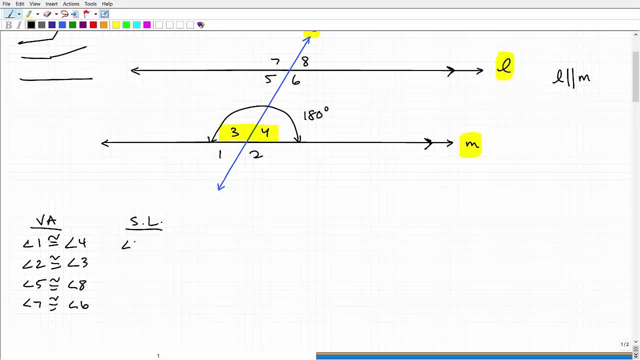 example, or supplementary, so we can say: angle 3 plus angle 4 is equal to what? 180 degrees? all right, now there's a whole bunch of these straight line relations relationships here. let me kind of erase this so you probably have already seen the many more. you probably say, well, seven and eight, five and six, one and two. 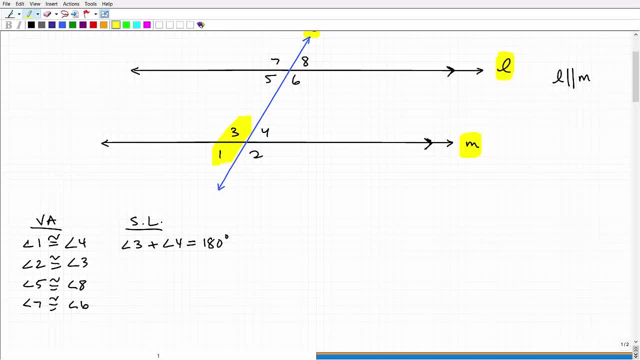 and you'd be correct, but also this way as well. one and three. okay, so one and three are supplementary. so angle one plus angle three is 180 degrees, and so forth. we can go on and on angle two plus angle four, 180 degrees, and so forth. we can go on and on angle two plus angle four, 180. 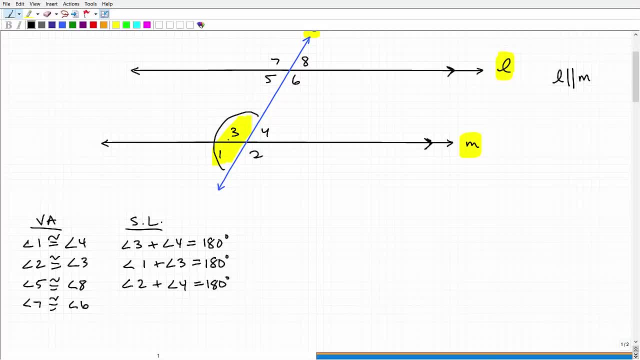 degrees and so forth. we can go on and on. angle three and four, angle one and two, angle one plus angle two is 180 degrees. five, six, seven, eight- actually I'm not going to list out the rest of them, but basically the same angles as we did in. 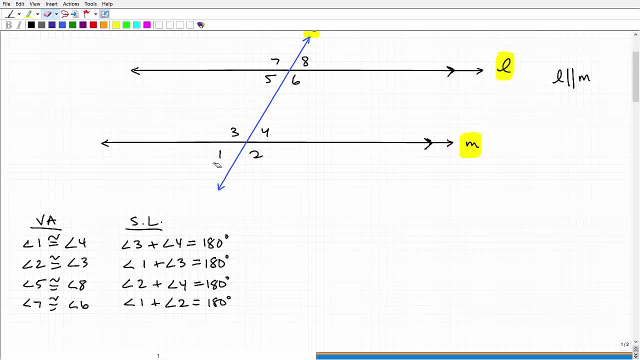 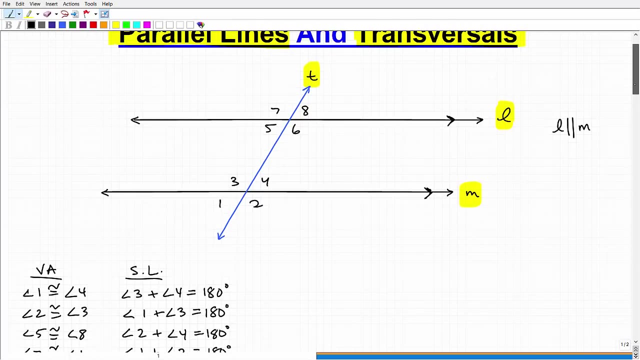 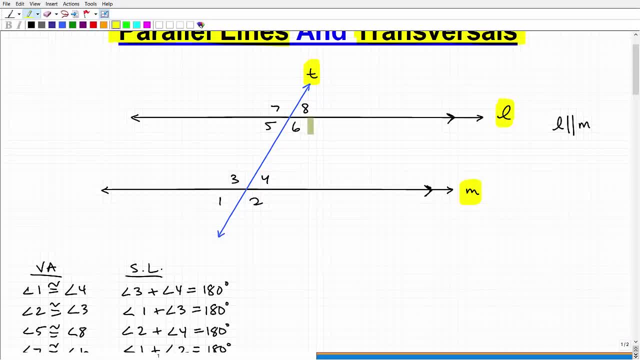 get into the next pair, want to kind of um, just denote a few things here. when we have parallel lines, we consider these angles here, these angles here- okay, inside the lines- as interior angles. okay, interior angles, so this would be exterior angles. these are a few points. interior angles, so these would be exterior angles. these are a few points. 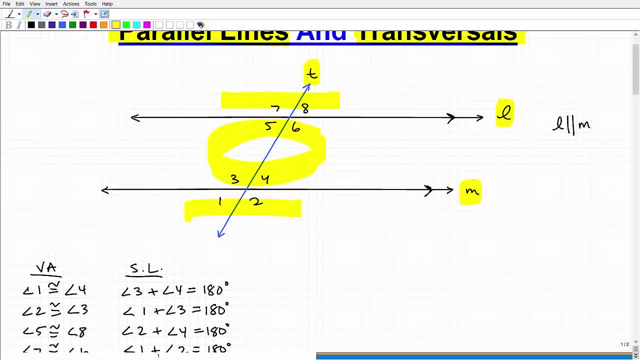 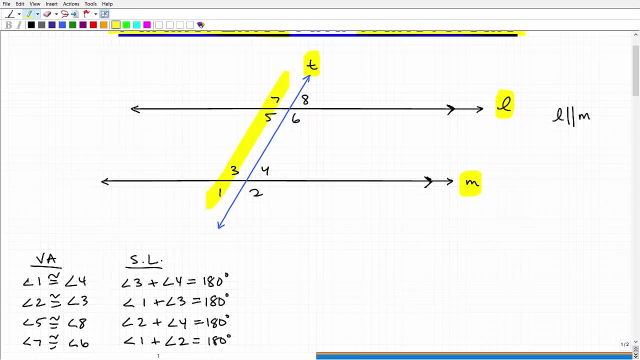 these guys here, but five, six, three and four would be considered interior angles. okay, so I'm going to be using the notation here, interior, and I'm also going to be using- let me just do it this way- that angles on opposite side of the transversal would be alternating. okay, that's that word, alternating. okay, so we 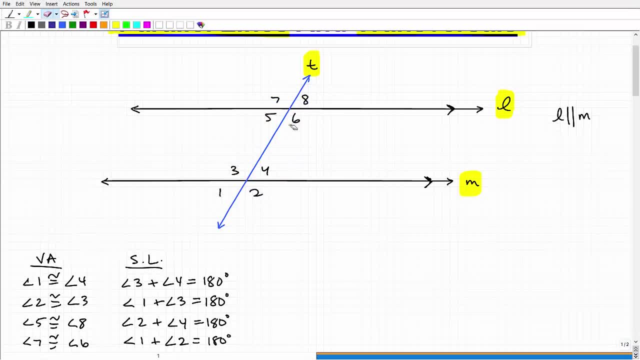 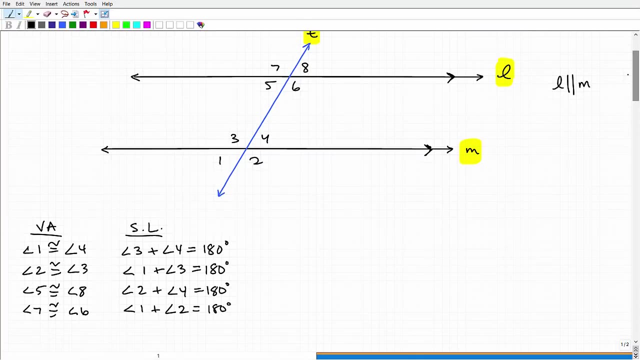 have interior and alternating, alternating our angles on our opposite side of the transversal, and interior are those angles that are inside the lines. okay, so what? that being said, kind of scroll down here a little bit, give ourselves some room. let's talk about the properties between angles five and six. 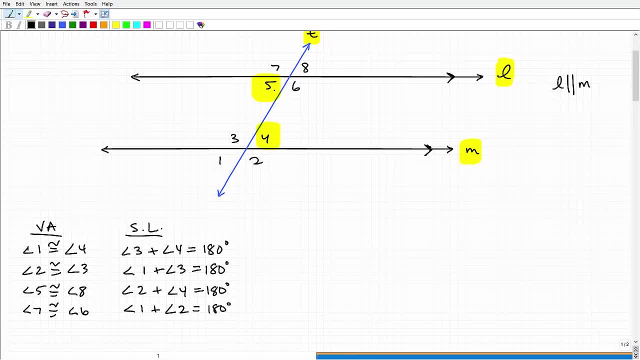 so what would we? how would we classify them? well, their interior angles and are alternate, also alternating angles. so we talk, we, we describe these as alternate interior angles. okay, so alternate interior angles. if you look here- angles five and angle six- they appear to be what congruent, the same angle. if 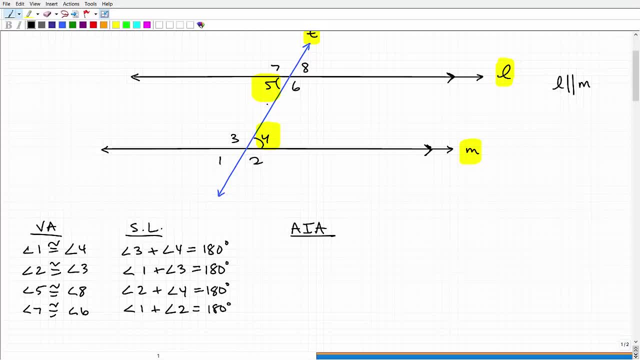 you kind of look at them closely and in fact they are. now, this is only true if these two lines are parallel, okay, if they're not parallel, then we can't make these um, these claims, okay, but in this case we can. so angle five is congruent to angle four and angle three is congruent to angle. 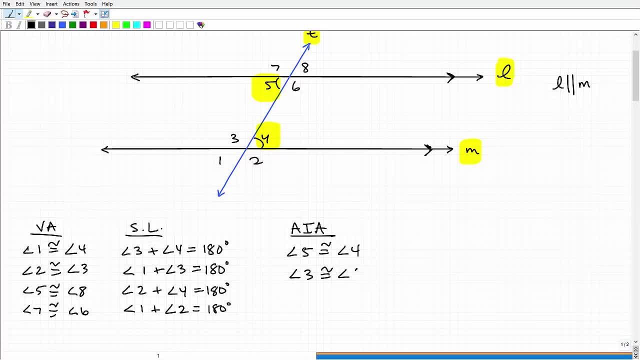 six. okay, why? because they're alternate interior angles and i'm going to give you some example problems here in a second, but let's just go and list all these out. so we have alternate interior angles. now we also have, let's say, these guys, what do you think we'd call the? 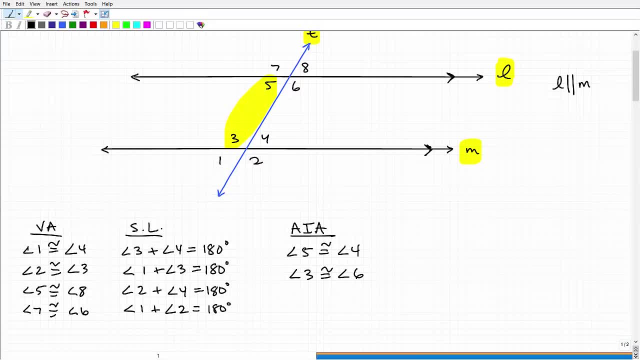 these pairs together, okay, what we call those same side interior angles. so same side interior angles. they have kind of a unique relationship. so let's say angle three plus angle five. the deal with these guys is they are supplementary. they add up to 180 degrees, okay. so angle four and angle six, all right, those are also same side interior. 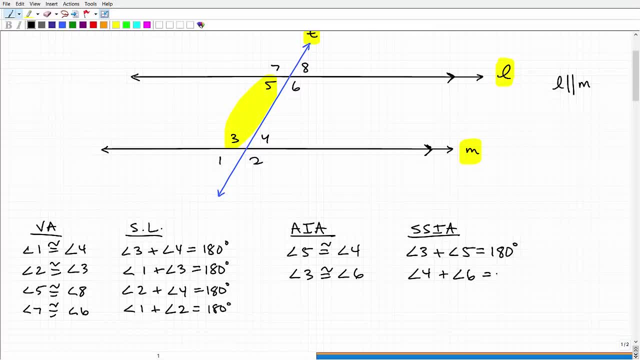 angles: angle four plus angle six, and they also add up to 180 degrees. okay, so let's just quickly review what we got so far. we got vertical angles, straight line angles, alternate, alternating- uh, interior angles, and we have same side interior angles. okay, and now we have another angle relationship and that is going to be corresponding. 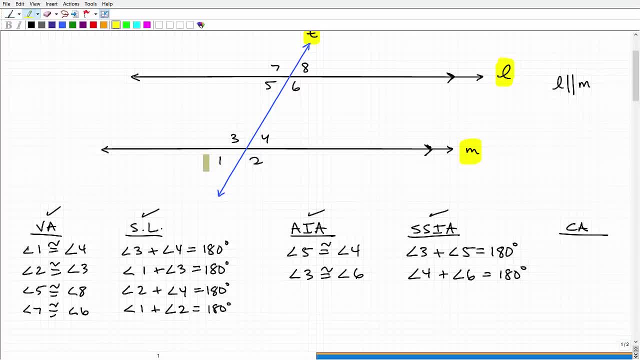 angles ofağı. so corresponding angles. so corresponding angles are pretty cool. what they they look like is this: let's take a look at angle one. so can you find another angle that looks like angle one? pretty much looks like the same angle measure. well, if you look kind of closely here. 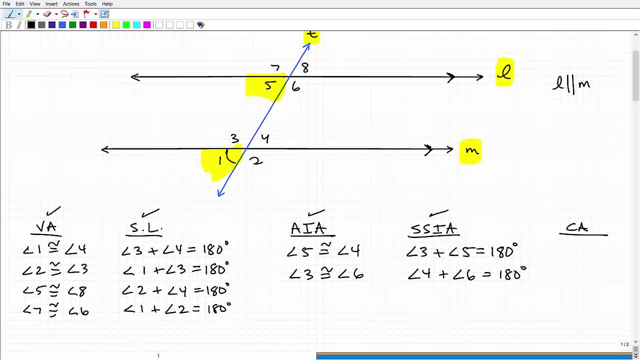 angle five does okay. so it's kind of like in the same relative position if you kind of look at it. this kind of corresponds to this well corresponding angles. again, all of this is predicated that the two lines were that that the angle is being formed, two lines that are parallel and are transversal. so everything I'm stating 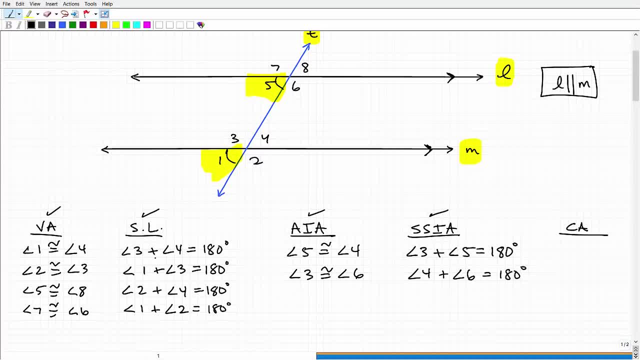 here, with the exception of vertical angles and straight line angles depend upon the two lines being parallel. okay, so corresponding angles are congruent. so that would be angle one. there's a whole bunch of these guys. angle one is congruent to angle five, and let me just stop here again. I know I'm kind of 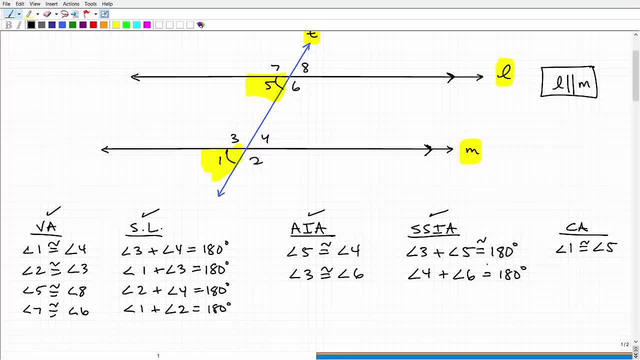 interjecting. here we use the word congruent. actually I got to put the word: well, no, equal to 180, that's fine. congruency and geometry is meaning that that we don't like to use the word equal. well then, you kind of use it. but 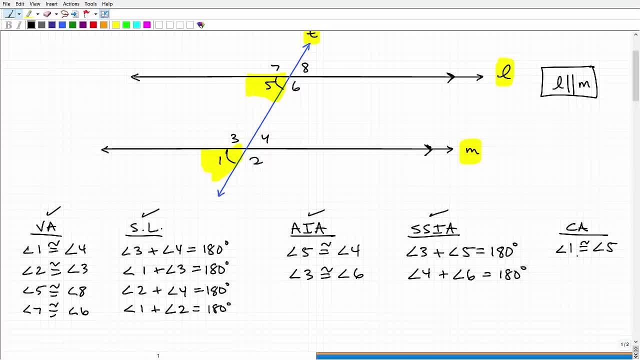 technically you're supposed to be congruent. that means they have the same angle measure. okay, where the equal sign is- usually when values like in algebra, like x equals 3 or something like that, then we'd like to use the equal sign. but we're talking about angle measure or the the length of segments, then you need to. 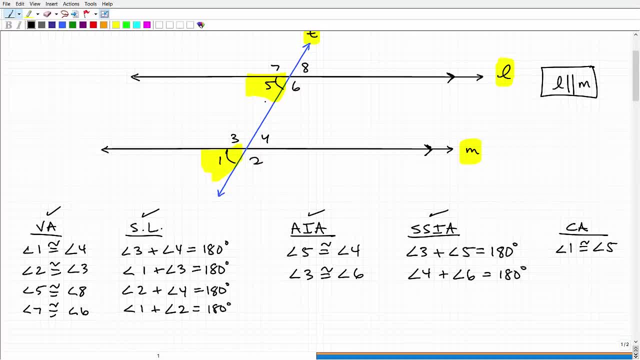 use the angle measure, and then you need to use the angle measure and then you use the, the congruent symbol. okay, so angle one is congruent to angle five corresponding angles, and then we can see three and seven. got a whole bunch. let's go list them out here and go: three is congruent to angle seven, and then on. 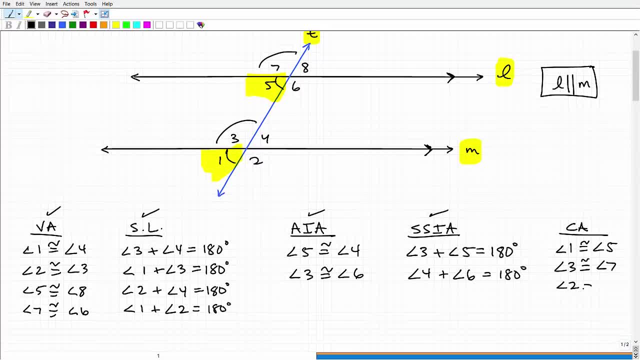 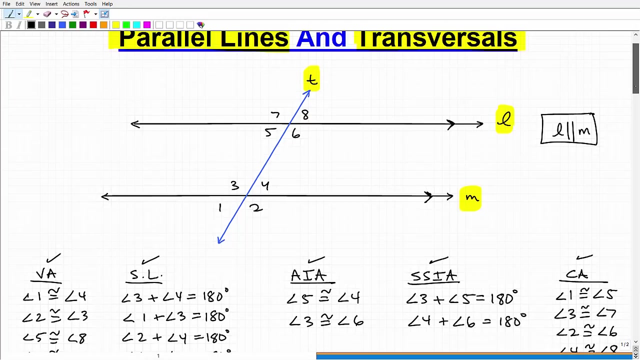 this side we have angle two is congruent to angle six and I see your angle four is congruent to angle eight. okay, I think that pretty much covers most of the angles being formed here. okay, with parallel lines and a transversal. all right, so knowing this, 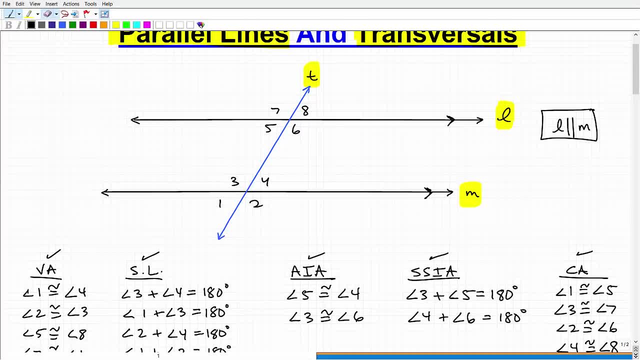 let's take a look at kind of like a typical kind of problem that you're gonna see in your geometry course or on any other type of exam. okay, so I suppose, pose, I'm given. let's say a, B, C, D, E, let's call this 30 degrees, let's call this Y and let's call. 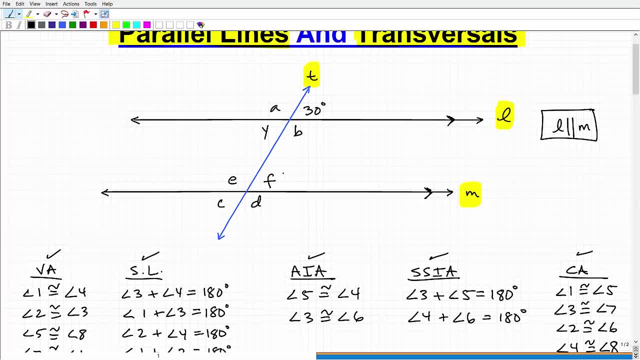 this F. okay, so you might be asked to find all the angles here. okay, all the value of the variables. so you're saying, well, I only got one angle here, but it's actually pretty simple. okay, so let's just start with angle a. okay, so how can we find the value of this guy right here? well, pretty, 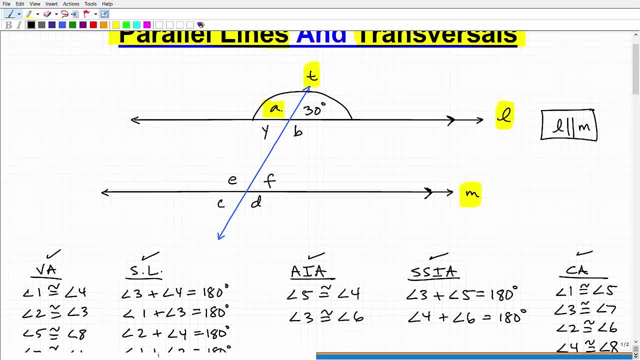 simple. actually, the way you can think about it is that these two guys angle. a plus angle 30 is equal to what it's a straight line angle. that's equal to 180 degrees. so a plus 30 is equal to 180. you can solve this basic equation. so a is equal to 150. okay, 150 degrees. it's very simple, right? so this: 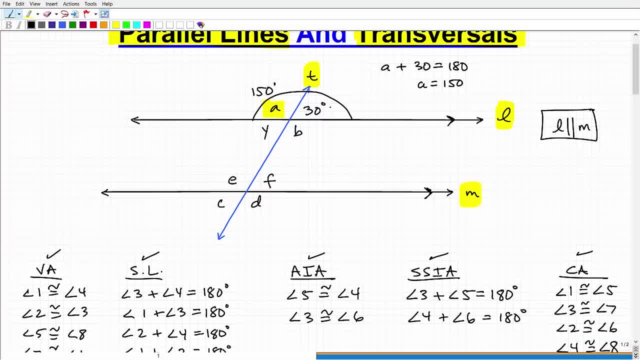 is 150, because 150 plus 30 has got to make up this entire straight line. so not now, knowing that you can be like, okay, these two are vertical angles, right here, these two right here are vertical angles. so B must also be equal to 150. okay, but Y because the vertical angles, and so is Y, Y and 30 vertical. 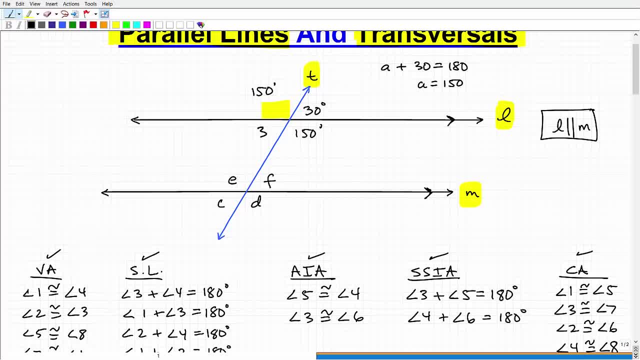 angles, so we can put a little 30 degrees right here and now we could just keep going down the line. so we got 50 right here. well, E angle E and 150 are corresponding angles, so this has got to be 150, and C and 30 are also corresponding angles and there's a different ways you can actually. 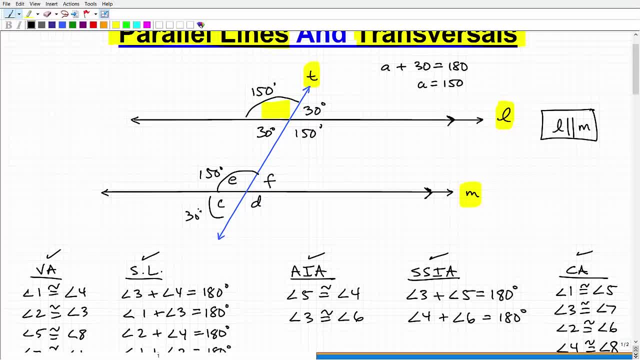 approach these. there's a ton of different- uh you know options, sometimes not all the times, but properties that you can use to apply here. and then E and D are vertical angles, so this has got to be 150. C and F are vertical angles. this has got to be 30 D and these are corresponding. and then boom. 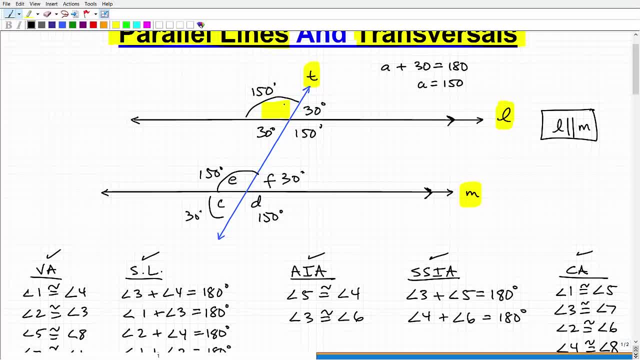 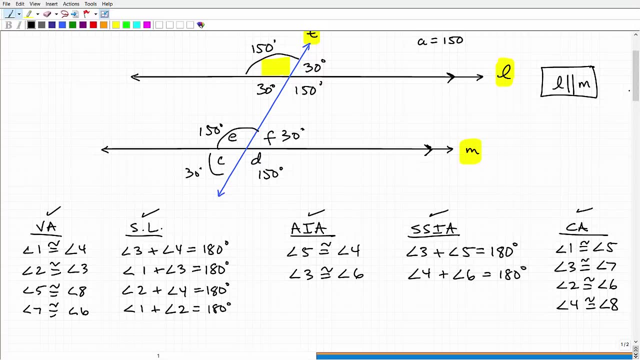 there, you're all done now. sometimes they'll have like like fancier algebraic expressions in there. you might have to set up equations, but this stuff is really not that difficult. if you know how to do basic, solve basic algebra equations and, most importantly, understand the angle relationships, you can get these problems right. but um a couple things again to stress. 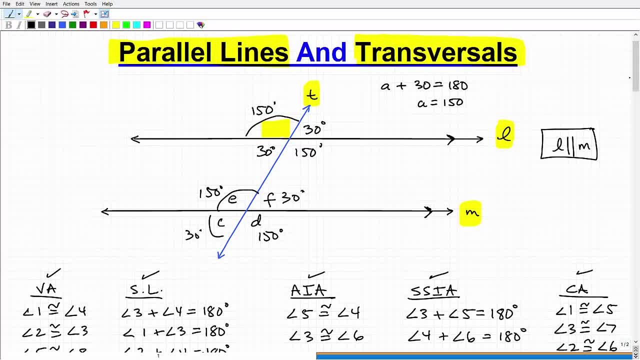 especially for those of you that are are taking tests, as I've seen this, definitely like on the SAT or the ACT, they'll try to kind of fool you that say the figures look to be one way, but in fact they draw the figure to kind of mislead you.